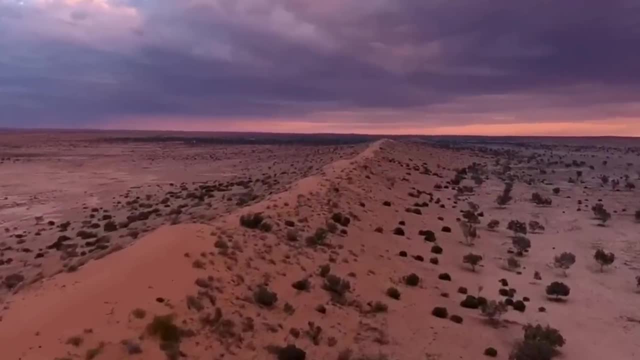 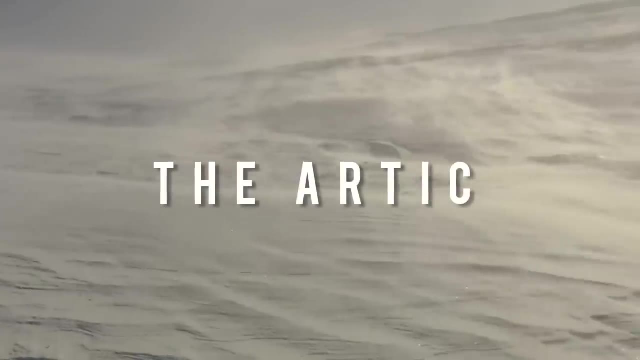 Australia is the driest inhabited continent on planet Earth and it is home to the Great Australian Desert, which is the fourth largest desert in the world After the Antarctic, the Arctic and the Sahara. Australia is comparable in size to the United States, However, its 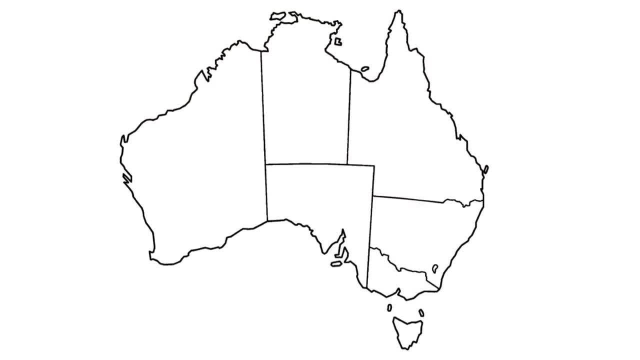 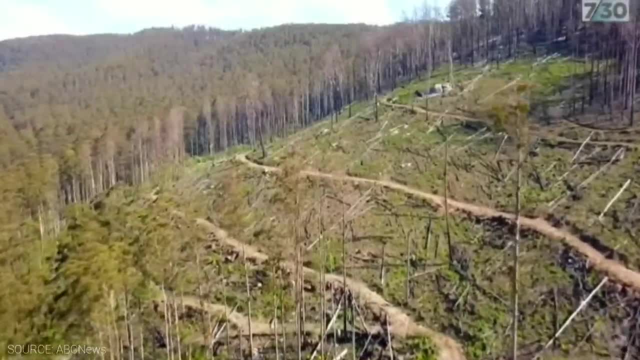 population is significantly less than America's. The whole of Australia has about the same number of people living in it as the state of Texas. Despite the low population, Australia is one of the worst developed countries in the world for broad-scale deforestation wiping. 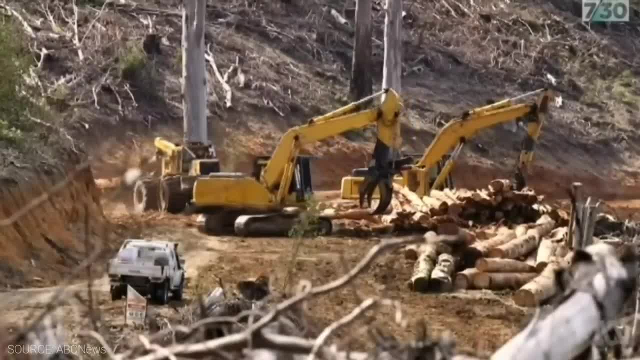 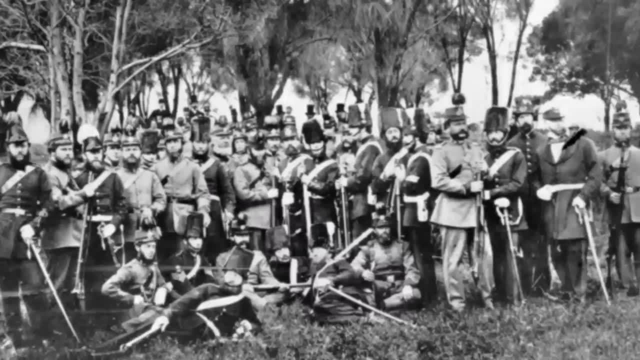 out endangered forests and woodlands. In fact, they have cleared nearly half of all forest cover in the last 200 years. It began around the early 1800s, when the British colonized Australia in search of land and fortunes. At that time, Britain had already been completely. 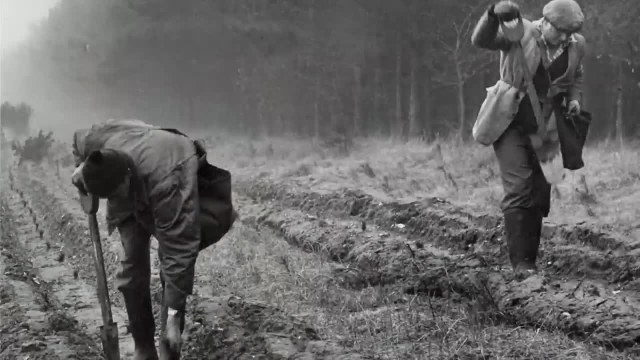 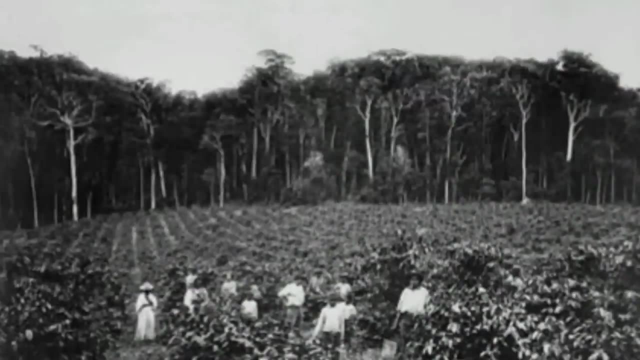 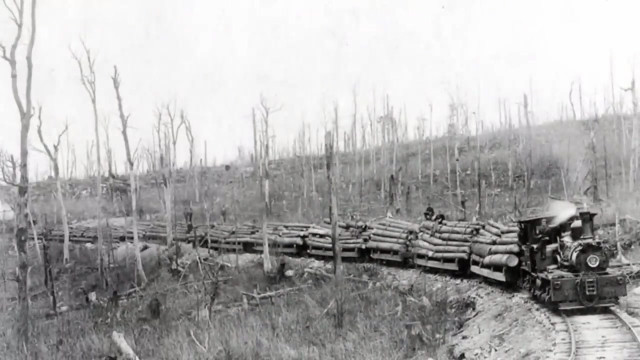 stripped of trees for centuries by intensive agriculture and war. Even today, the United Kingdom has one of the lowest percentages of forest cover in Europe. British timber companies were granted free access to vast areas of virgin forest in Australia, and trees were felled for agriculture and railway tracks, which were constructed alongside other transit. 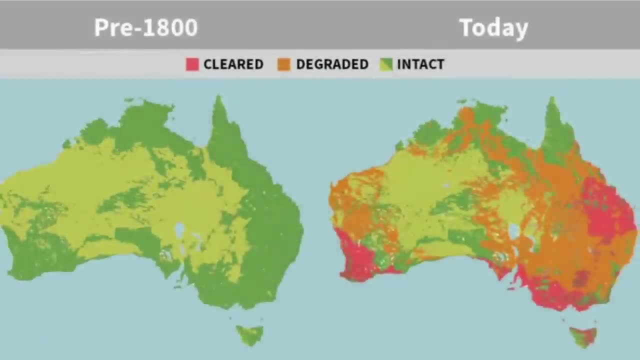 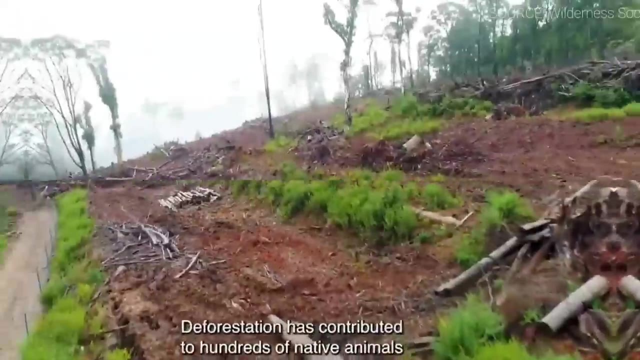 infrastructure such as roads, bridges and jetties. By the 1880s, concerns about stripping the forest were being raised, but no steps towards conservation were taken, And now Australia has become the worst offending country in the world for mammal extinctions- 55 wildlife. 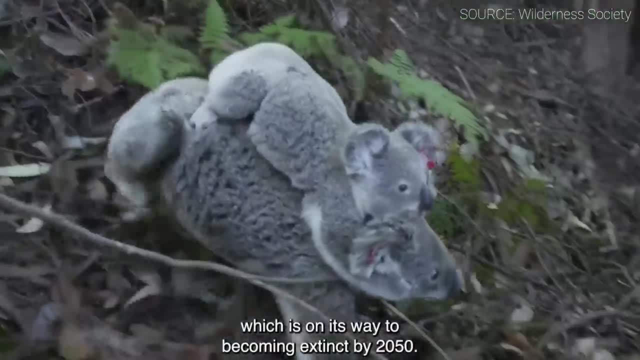 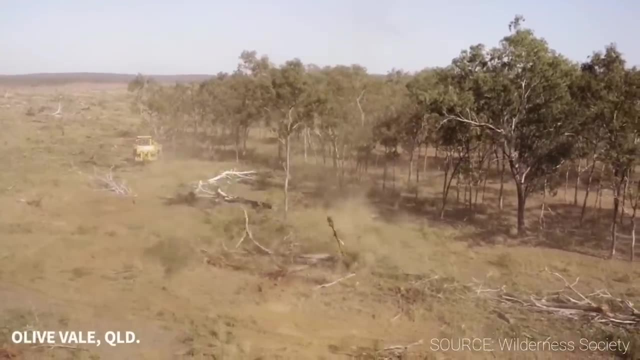 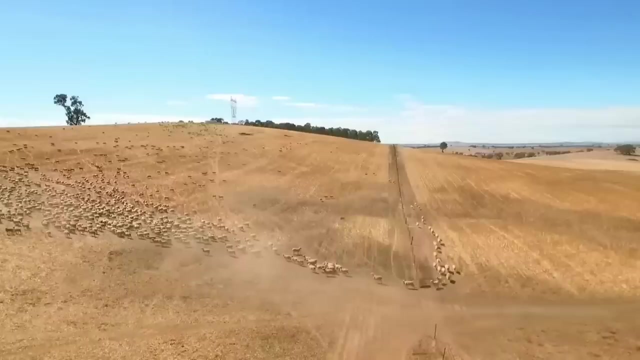 species, plus 37 plant species, have gone extinct. The widespread deforestation has resulted in 55% of all Australian land area being used for agricultural purposes and around 72% of all agricultural output is exported. Meat and live animals has been the fastest-growing export segment, growing 33% in value. However, agriculture only accounts for 1.9% of the value-added GDP and 2.5% of all employment in 2020 and 2021.. The widespread land degradation has resulted in man-made desertification after centuries of tilling and the introduction of non-native grasses has taken its toll on. 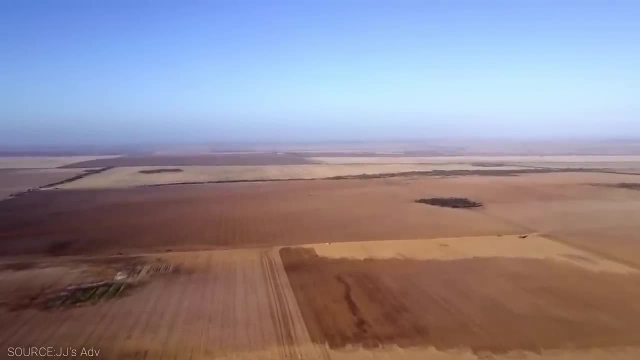 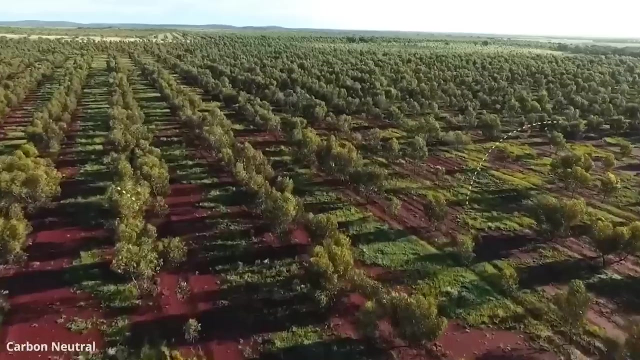 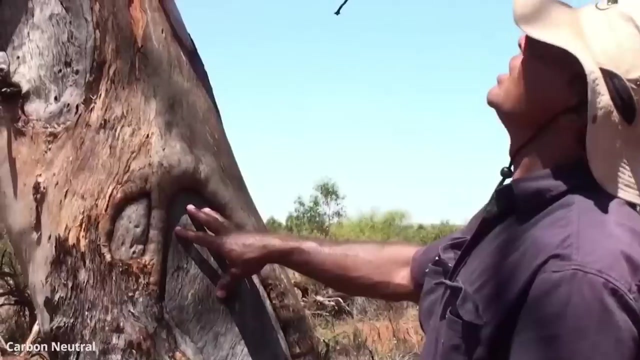 the landscape. However, some regions in Australia are starting to turn this around, transforming large areas of degraded land back into biodiverse ecosystems By restoring millions of trees and, in turn, improving the lives of rural farming communities, as well as capturing over a million. 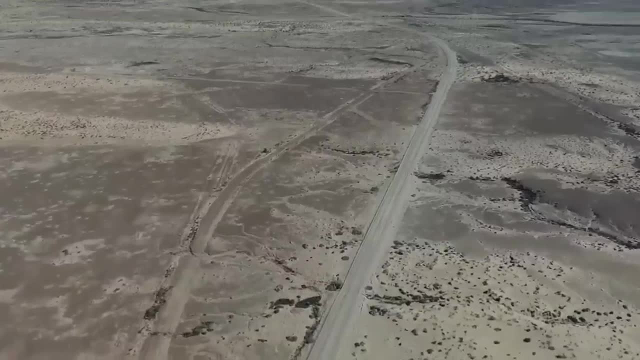 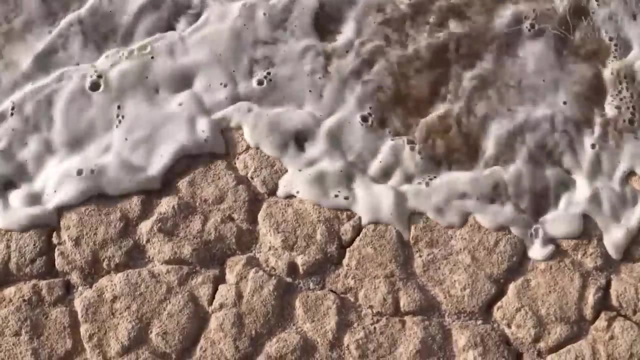 tonnes of carbon to benefit the planet as a whole. this can be considered a major accomplishment for any country, particularly one that has a low average rainfall of 16 inches per year. In this video, we will show you how a 200-kilometre-long green corridor will connect 12 nature reserves. 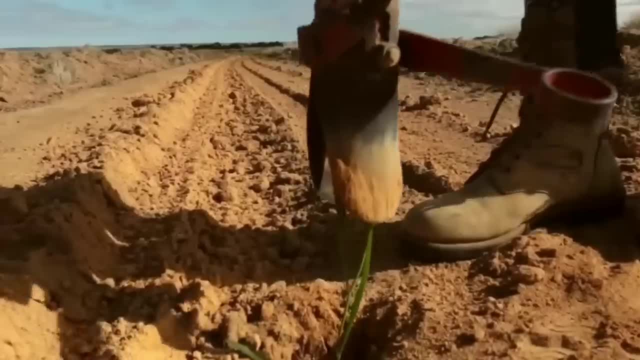 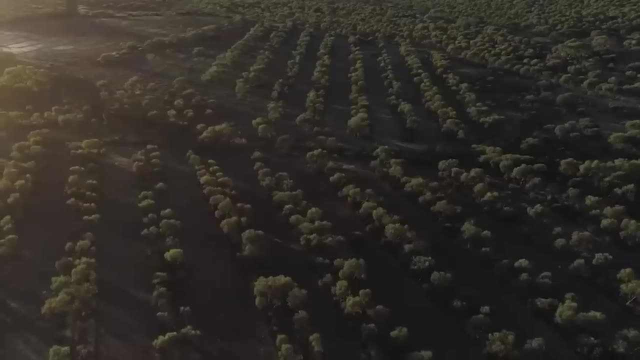 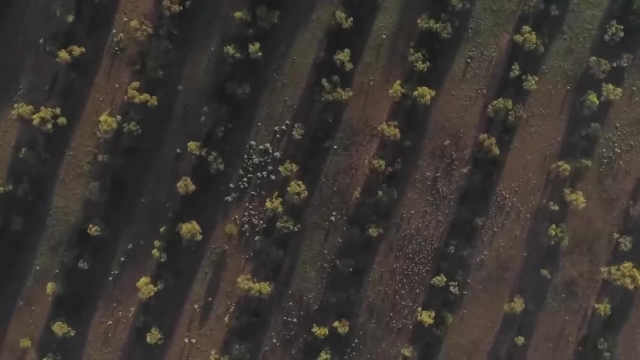 across 10,000 square kilometres. so stick with us as we dive into today's video. This large-scale reforestation project is in one of Australia's most vulnerable regions. Nearly 20 million trees across 10,000 hectares of degraded farmland have been planted, transforming 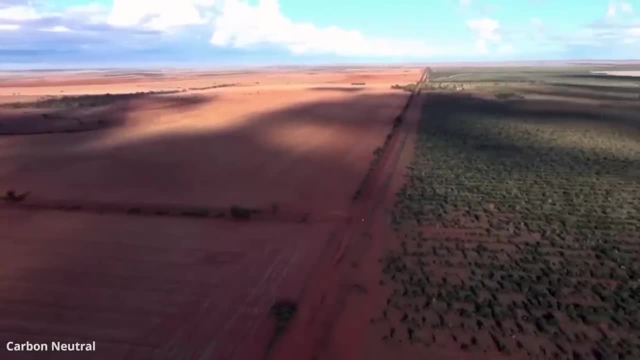 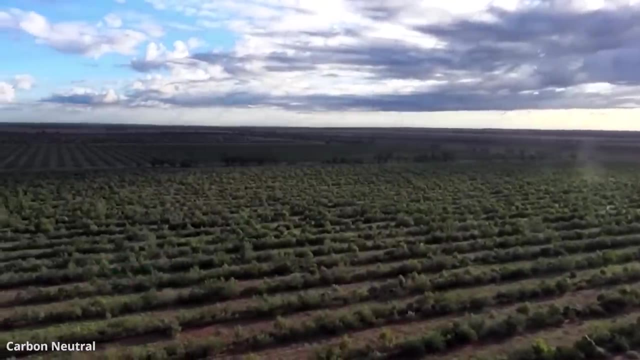 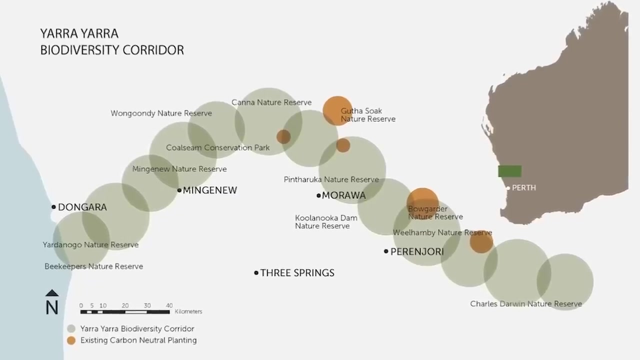 barren areas of parched earth. Carbon Neutral is a biodiverse carbon sink developer working on some of Australia's largest reforestation projects. This project is part of the Yarra Yarra Biodiversity Corridor in Western Australia's Midwest, connecting vital areas of land in the Yarra Yarra Biodiversity. 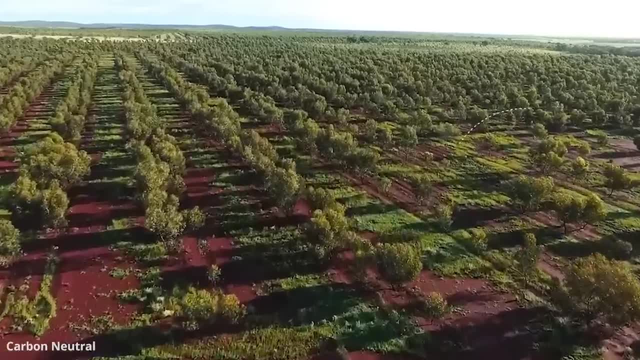 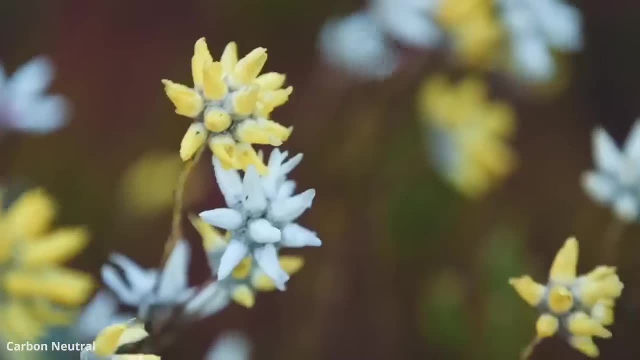 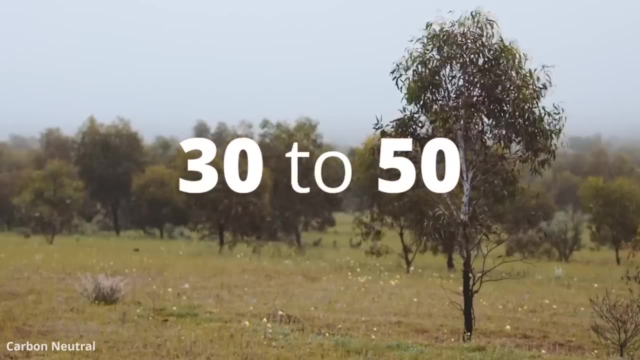 Corridor. Biodiversity corridors are areas of vegetation that allow animals to travel from one patch of native forest to another. A corridor provides shelter, food and protection for many predators by imitating the structure and diversity of native vegetation. The forests contain 30 to 50 different native species. All of the seeds are collected from. 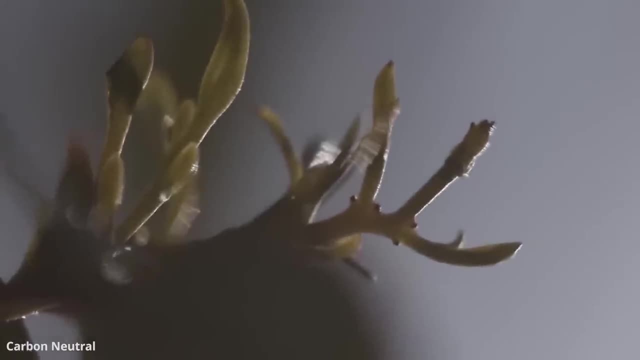 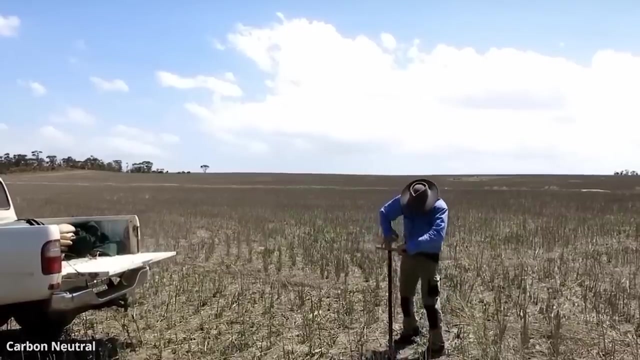 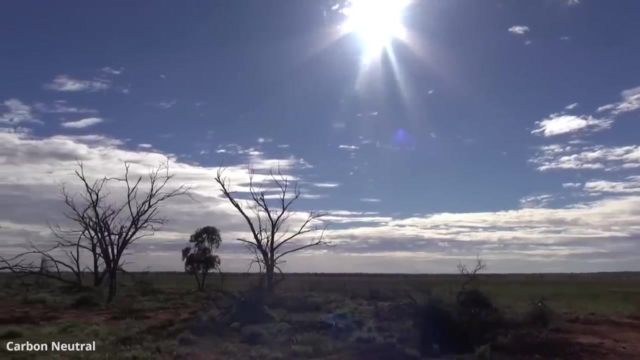 within 20 kilometres of the project area, ensuring they are located and adapted to the area, helping to restore the native biodiversity. Soil types across the project areas have been analysed so suitable species could be selected for planting. It reclaims a lot of salt land and is helping to prevent wind and water erosion. 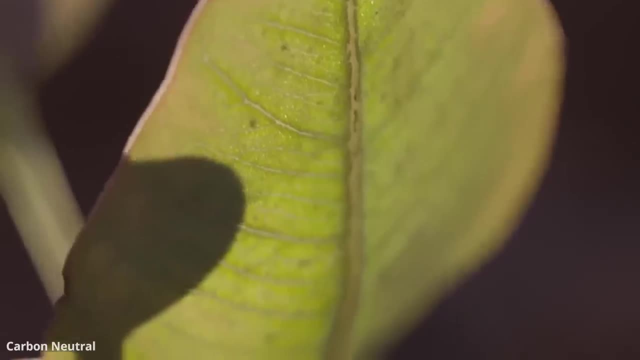 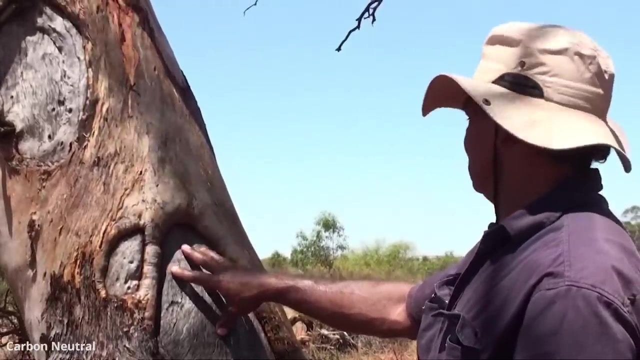 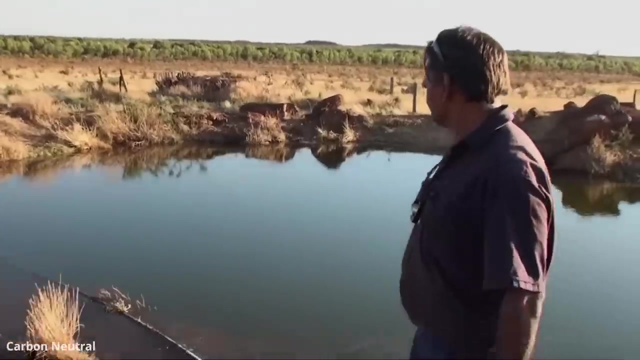 providing significant habitat for flora and fauna, including some of Australia's rare and endangered species like the Nallie Fowl and the Carnaby Black Cockatoo. The project aims to employ local indigenous people and is currently providing jobs for 10 people. Work includes helping with seed collection, fencing, land management and working. 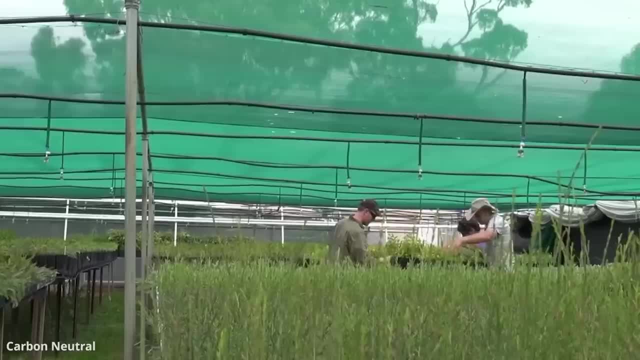 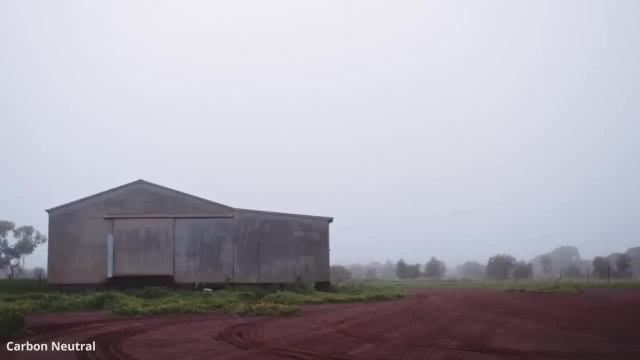 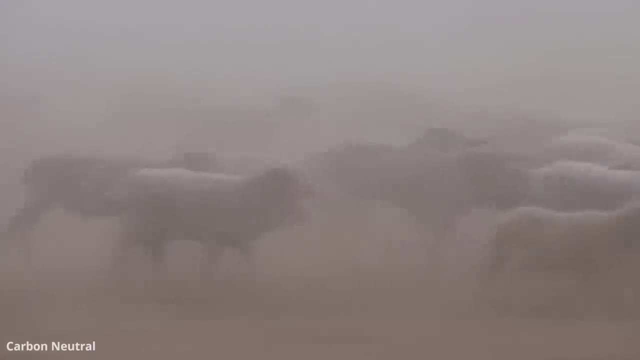 with traditional landowners throughout the region. 80 local businesses are involved and the project has cost AU$4 million. The project is situated in Western Australia's Wheatbelt, an area cleared for agricultural land, And intensive farming has caused erosion and degradation of the soil, devastating native